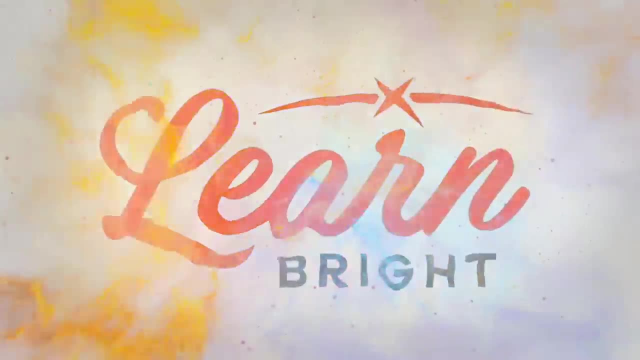 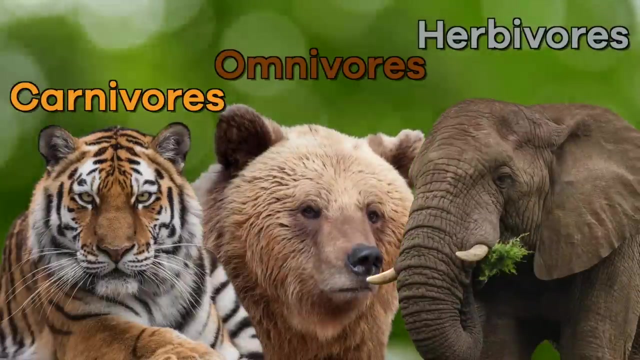 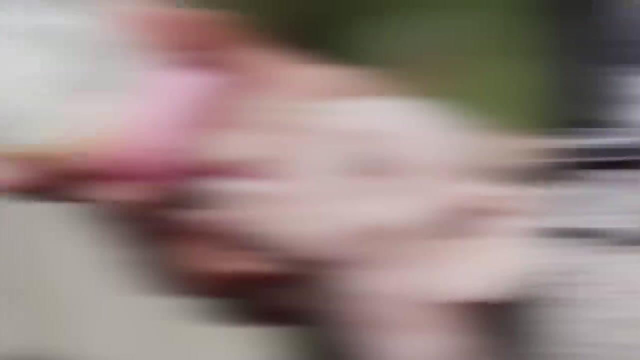 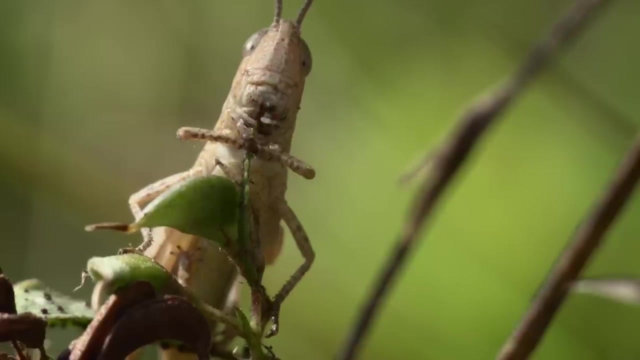 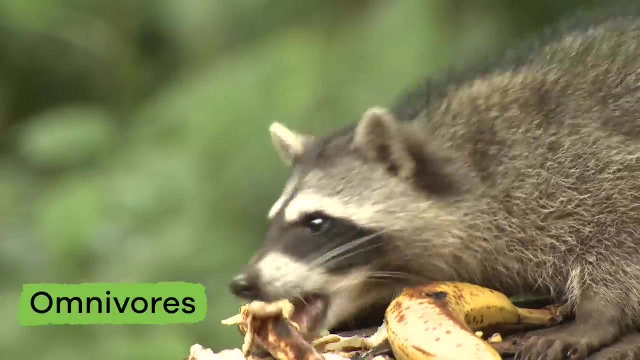 Herbivores, carnivores and omnivores. Every animal in the world has at least one thing in common: They must eat. But what animals eat can be totally different depending on the kind of animal. Animals can be herbivores, carnivores or omnivores. Today we are going to talk about 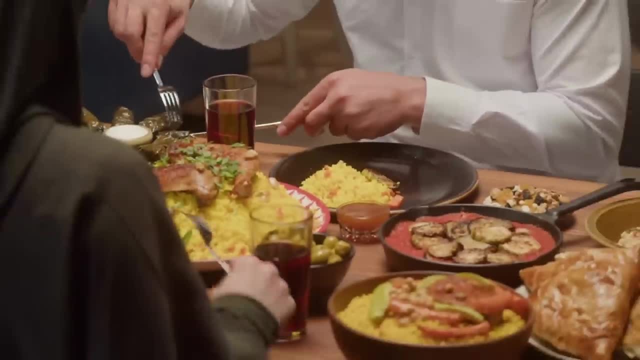 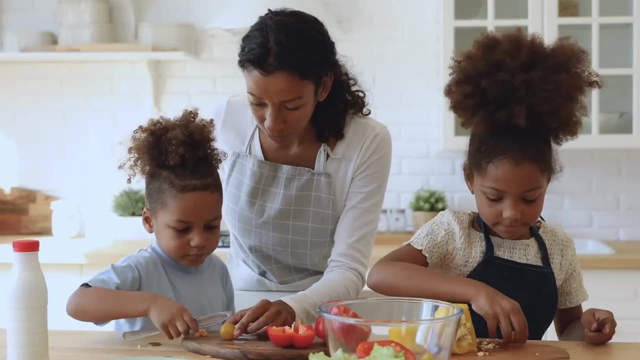 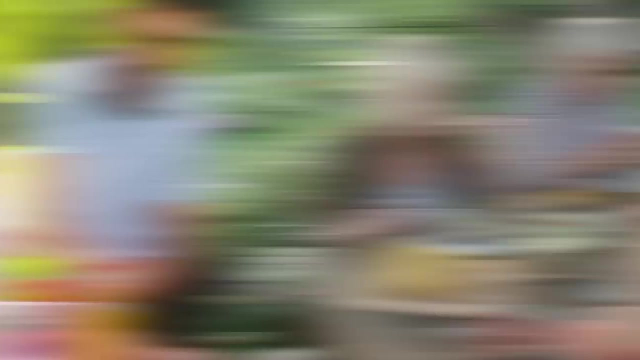 what each of these words mean. But first let's quickly pretend we are eating dinner together. What types of food do you usually eat? It might be a combination of meat, vegetables or fruit, Or maybe you do not eat meat at all. 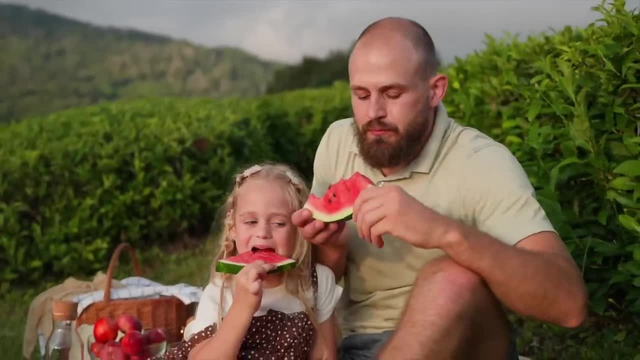 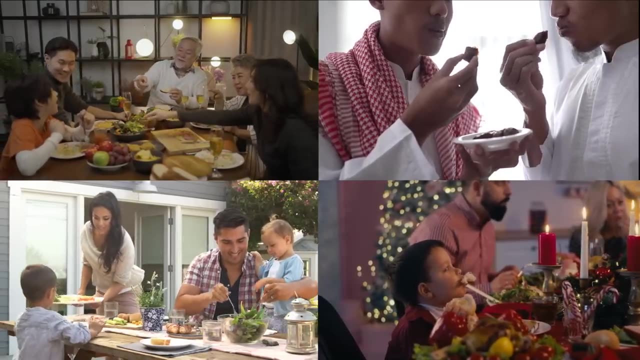 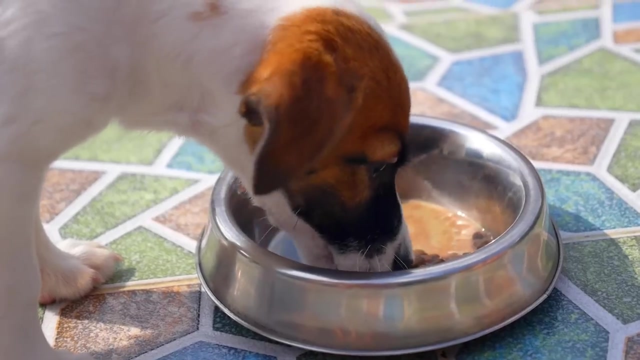 Or maybe you eat lots of fruit when you are not in the mood for vegetables. Not every human has the same diet or favorite foods, and neither do animals, So let's see what animals are having for dinner. We already mentioned that animals can be herbivores. 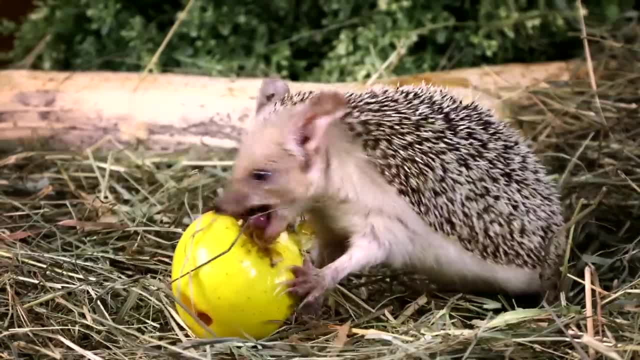 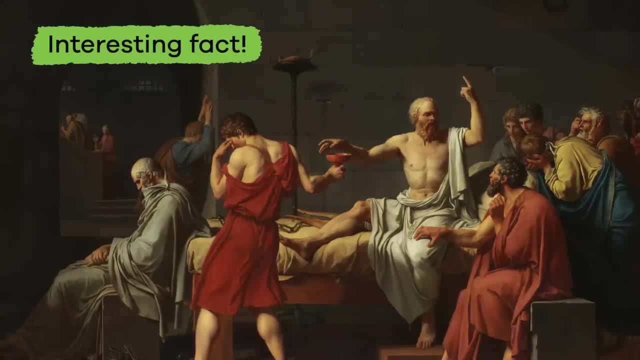 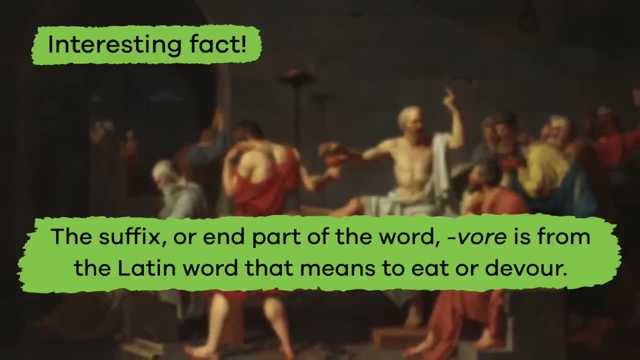 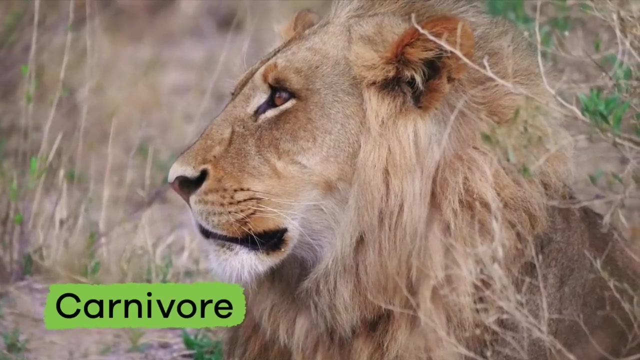 carnivores or omnivores. When you look at these words, what do you think that vor means? Here is an interesting fact: The suffix or end part of the word vor is from the Latin word that means to eat or devour. In this case, vor is combined with the prefixes or beginning parts. 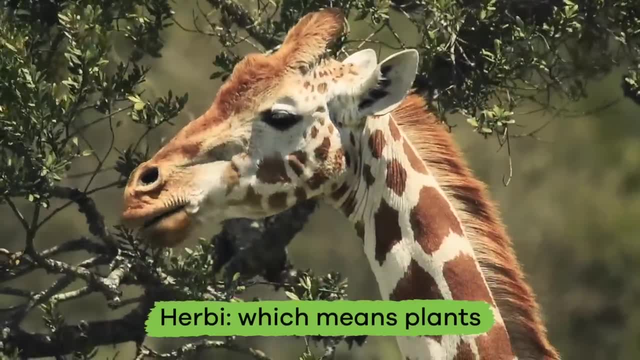 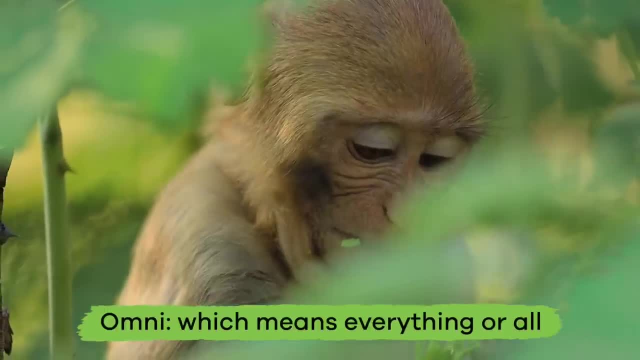 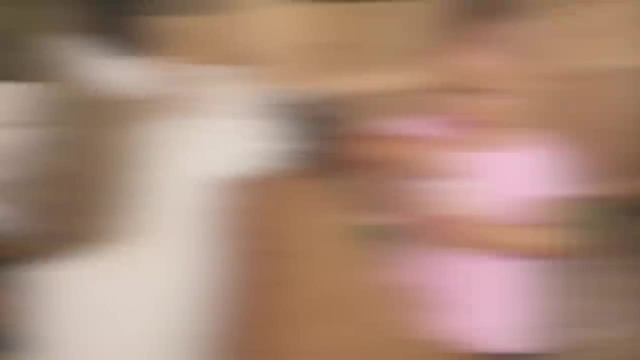 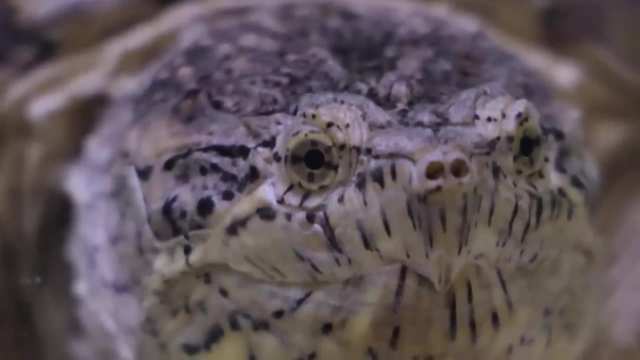 of the words herbe, which means plants, carne, which means meat or flesh, and omni, which means everything or all. Knowing the definitions of these words will come in handy. so keep them in your brains, Because now it is finally time to talk about these three cool animal diets. 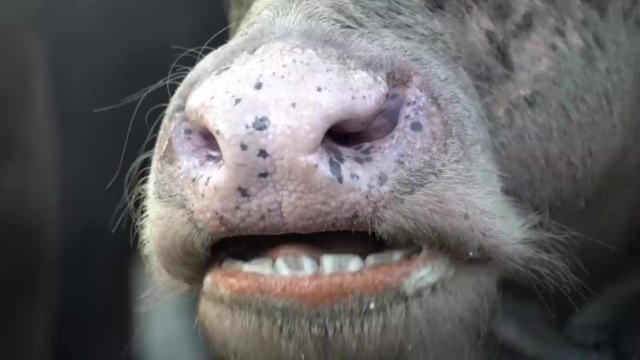 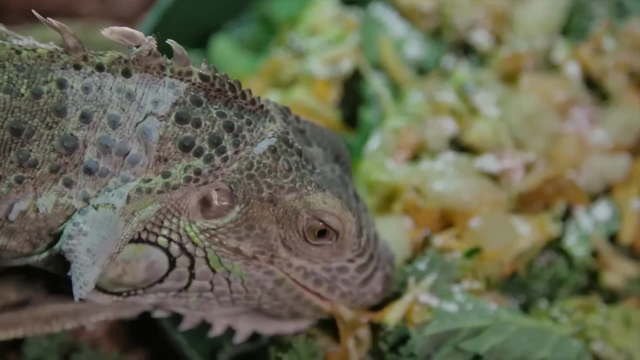 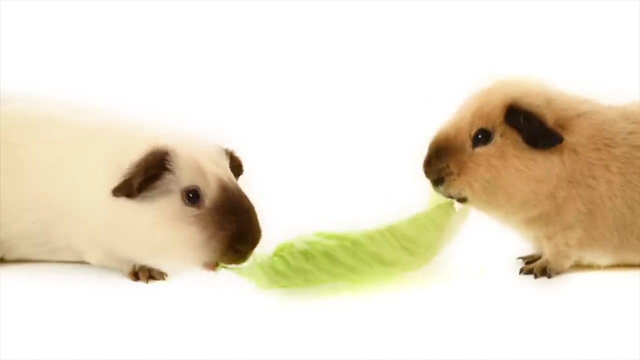 First up is herbivore. As you can probably guess, herbivores are animals who only eat plants. No meat for them, Not even when it's a juicy hamburger, Though they might eat the lettuce and tomatoes. Physical characteristics of herbivores include: 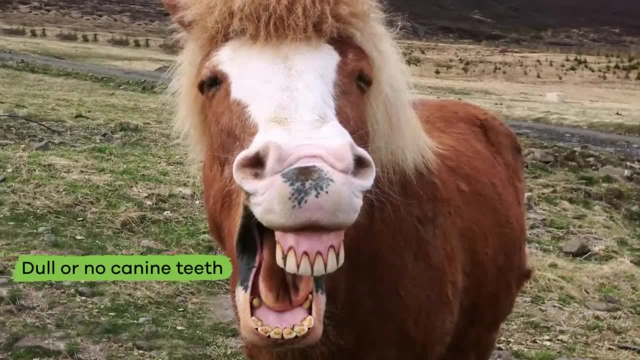 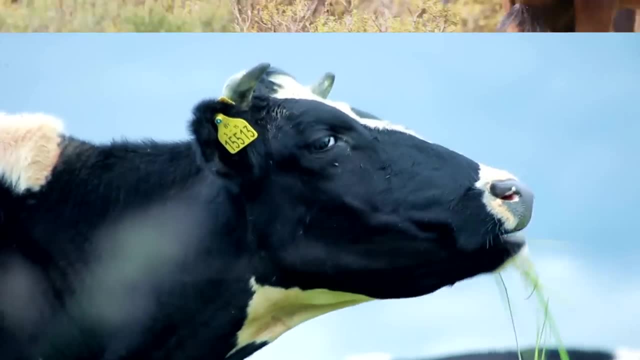 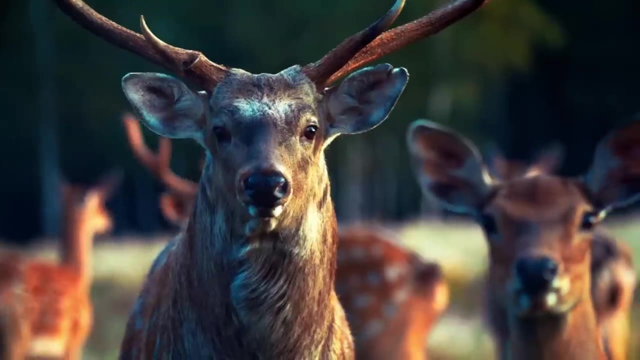 dull or no. canine teeth with big flat side and back teeth. Herbivores use their molars to crush and grind plants. The eye placement of most herbivores is located more on the sides of their heads Because they do not eat plants. 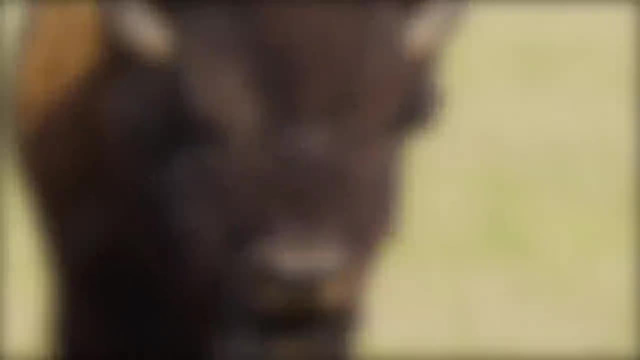 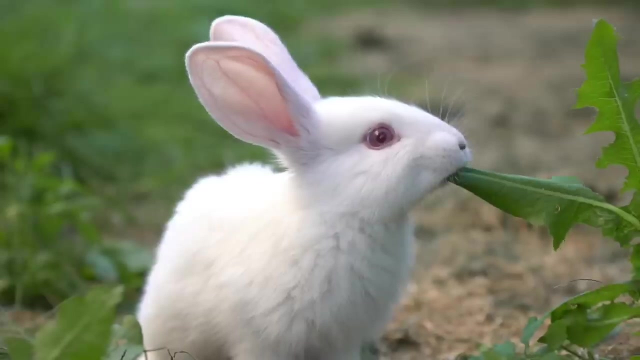 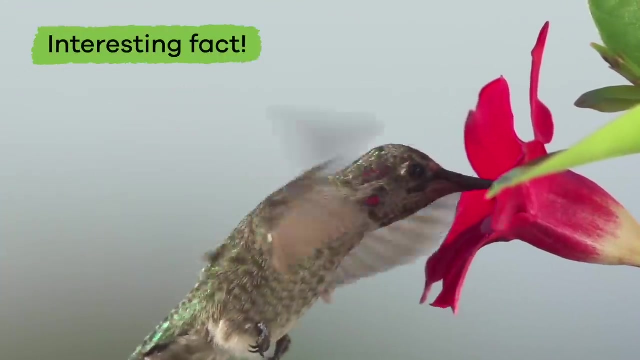 They don't have to track down or hunt prey. Not all herbivores are the same. Some eat only grasses, while others eat different kinds of plants, seeds or fruits. Here is an interesting fact: Birds, bees and butterflies eat nectar from. 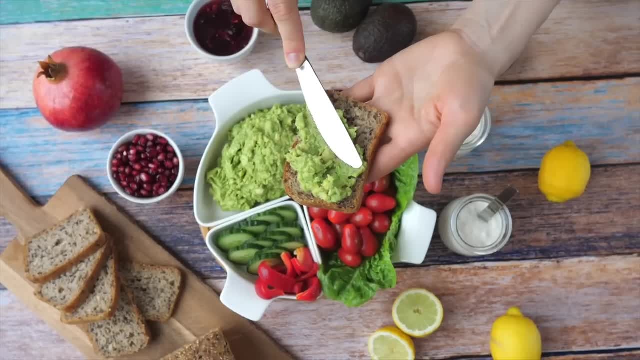 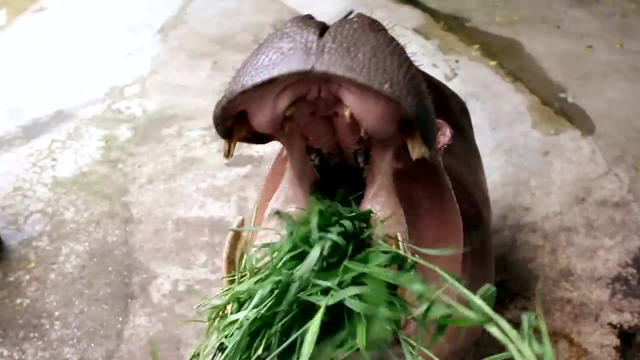 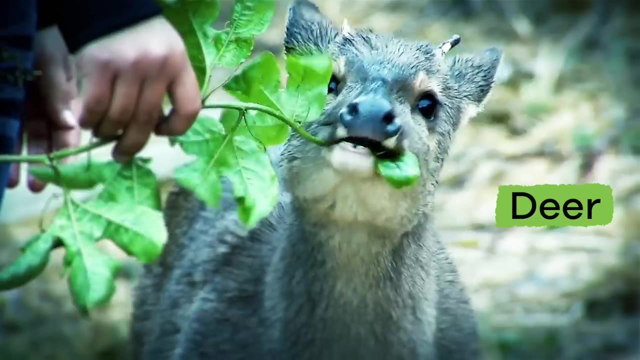 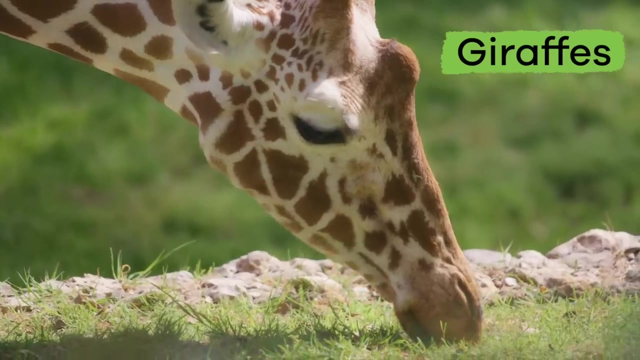 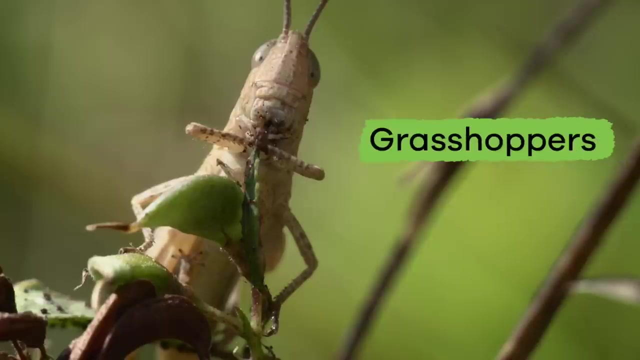 flowers to get the nutrients they need to survive In the human world. vegetarians are people who eat plants and do not eat meat, just like herbivores. Examples of herbivores are sheep, cows, deer, squirrels, elephants, parrots, giraffes, kangaroos, mice and insects such as caterpillars and. 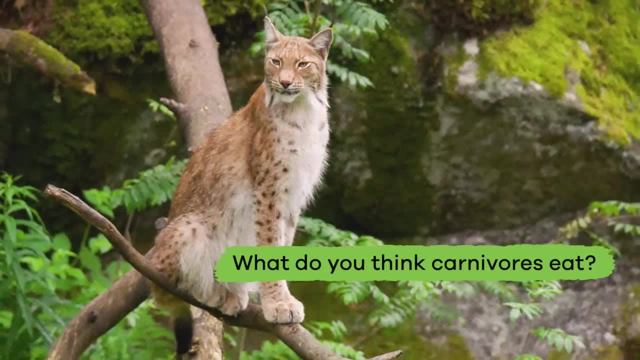 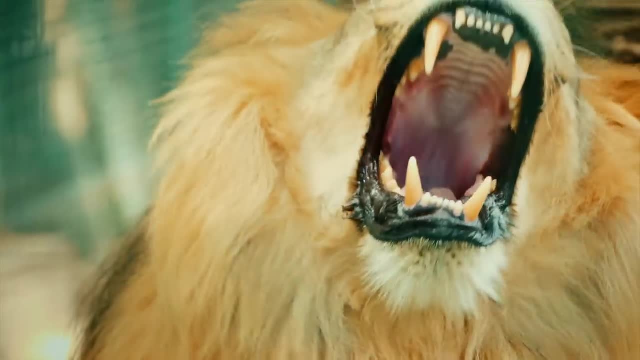 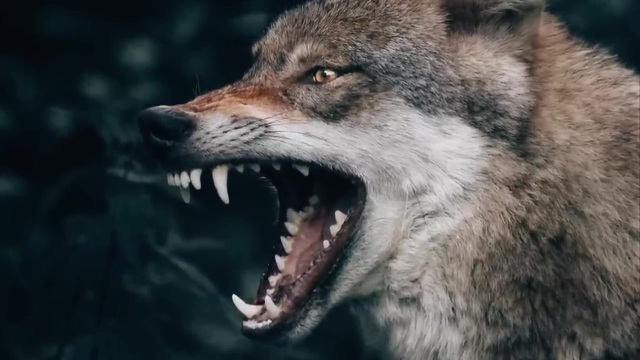 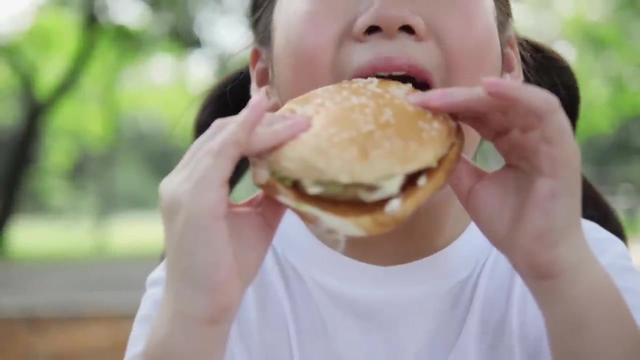 grasshoppers. What do you think carnivores eat? If you said meat, you are right. Carnivores are animals with long, sharp canine teeth next to their front teeth, plus sharp cheek teeth called carnesials. Try saying that three times fast. Bet they would love to sink their teeth into a juicy. 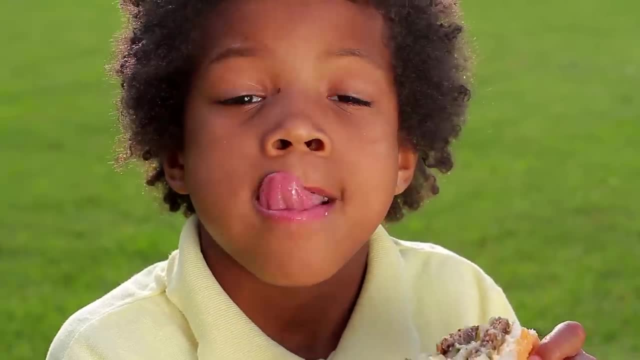 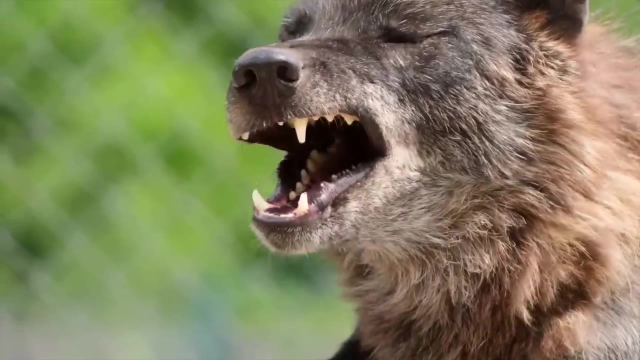 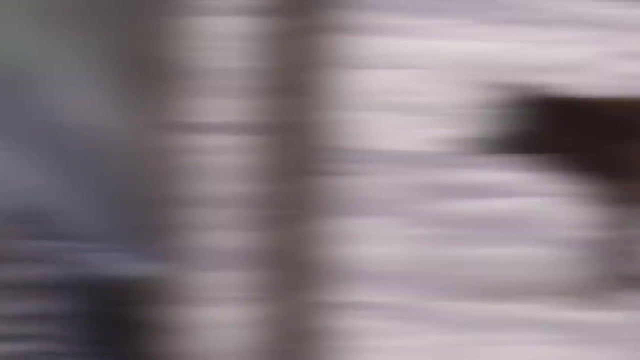 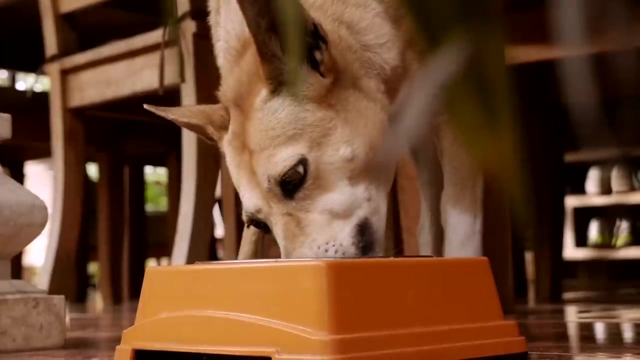 burger patty. These sharp teeth are perfect for seizing and stabbing prey and chewing them up. Unlike herbivores, carnivores' eyes are located in the front of their heads so that they can spot and determine the distance of their prey. Meat is a high-energy food source for carnivores. 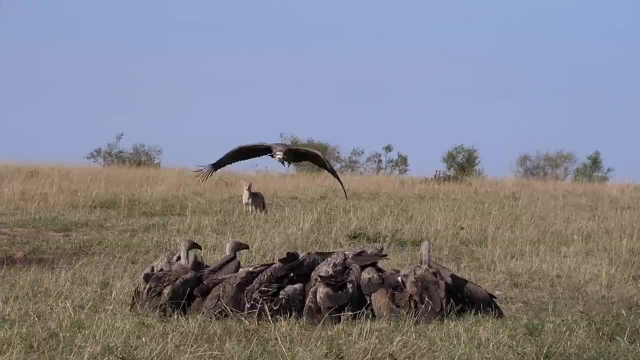 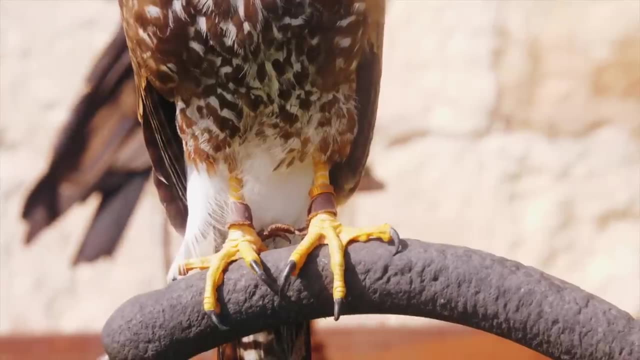 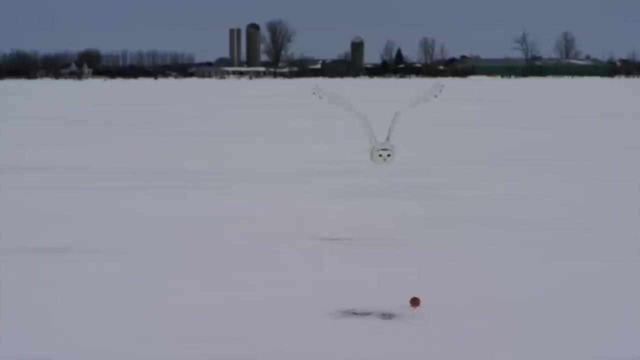 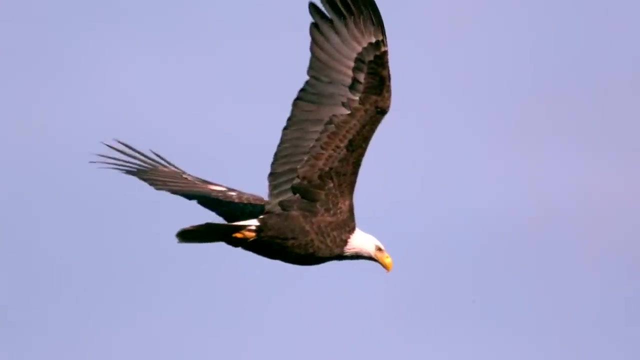 They find their food by hunting live prey or by eating animals that are already dead. Many carnivorous animals have big claws, sharp teeth or beaks and quick speed. This is all to help them hunt, whether they live on land, swim in the sea or soar through the sky. 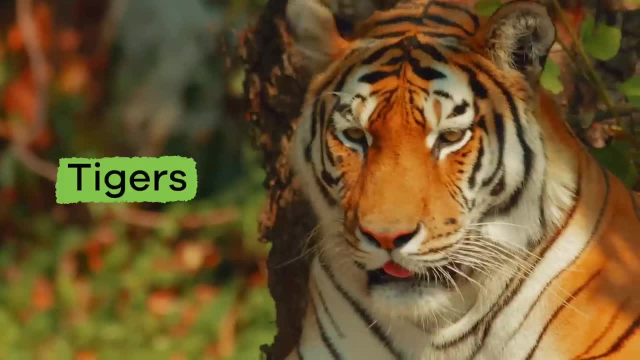 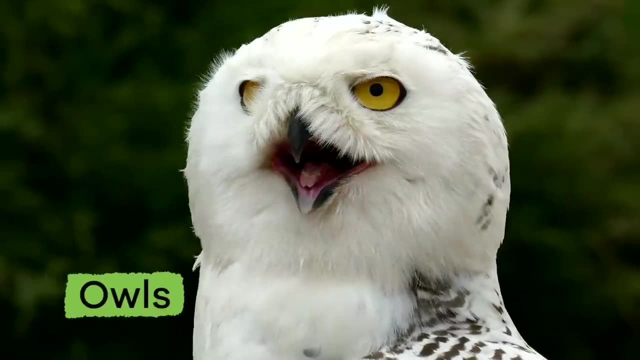 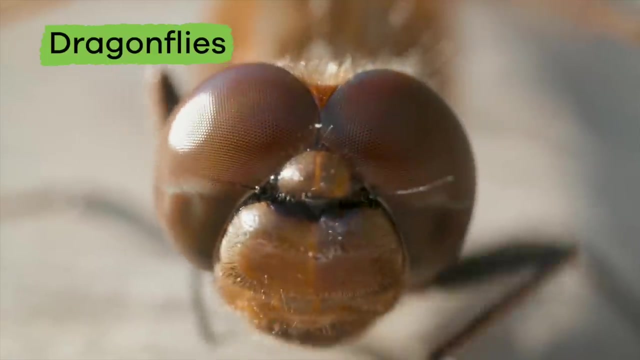 Animals like lions, tigers, crocodiles, wolves and snakes, Birds like owls and eagles, And insects like beetles and dragonflies are all carnivores. So is the venus flytrap, which is actually a plant. 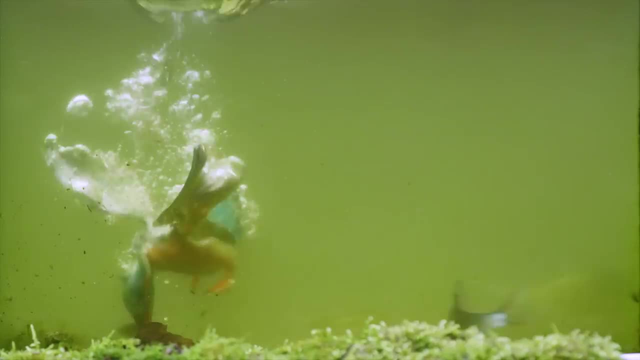 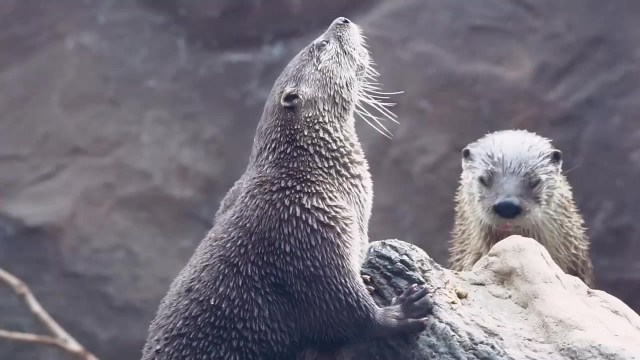 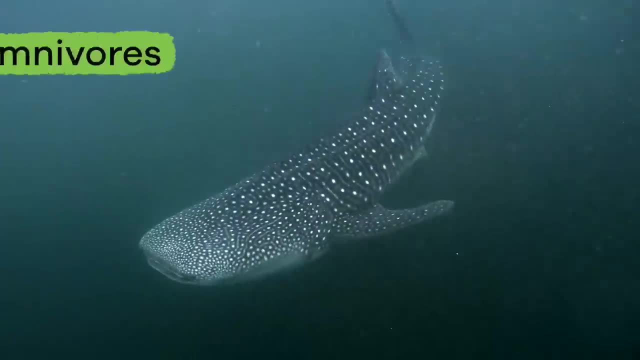 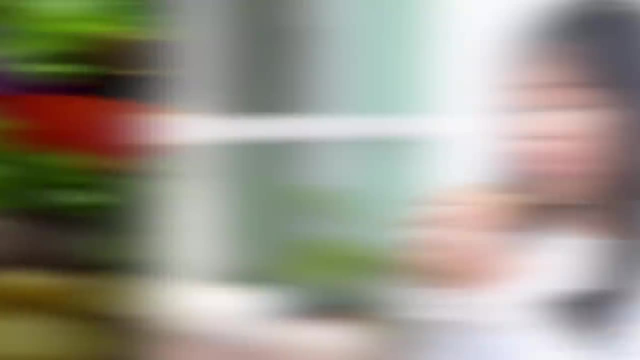 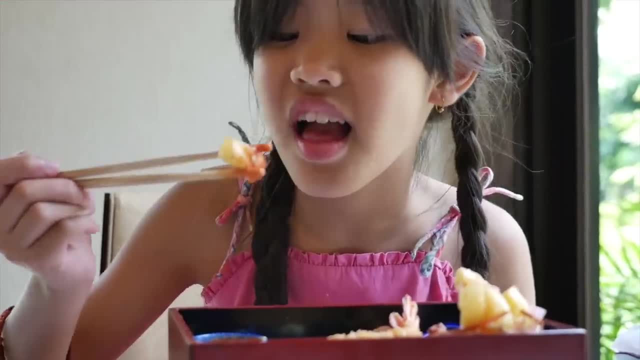 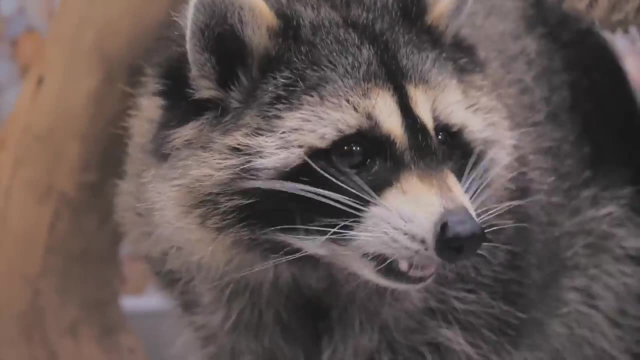 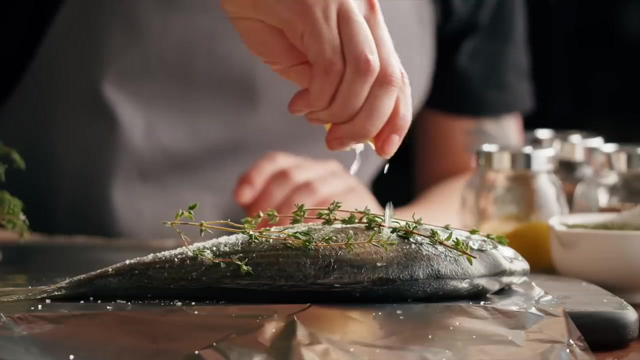 If the omnivore is a human, that is, In fact, most humans are omnivores. Like other animals, omnivores may limit the types of plants or animals they eat, Just like humans. Some humans might only eat plants and fish. 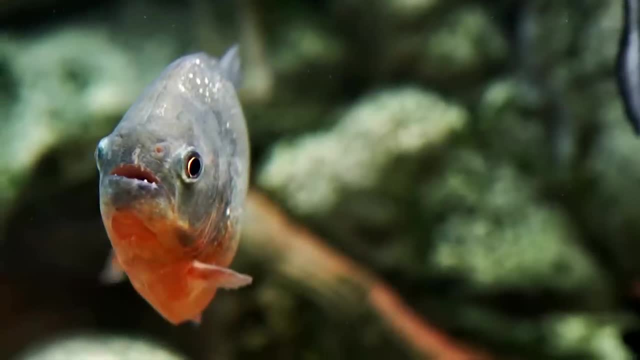 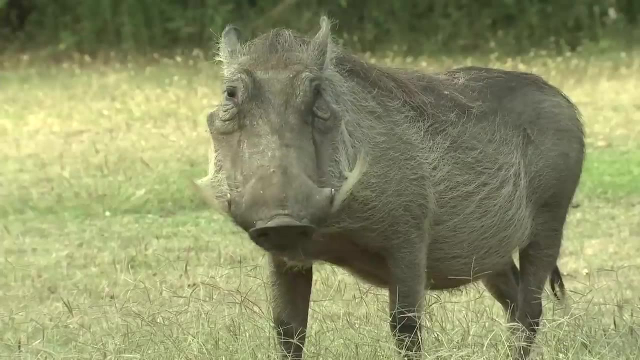 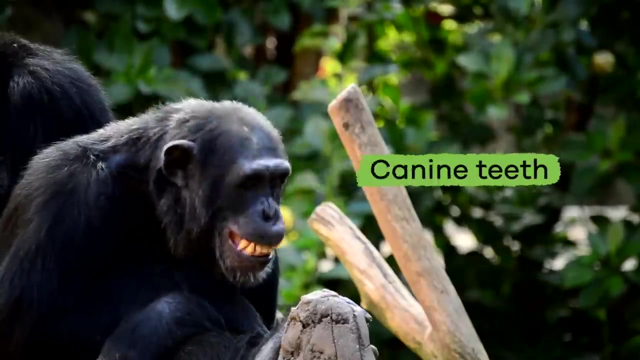 but no other animal products. Omnivores in the wild have the widest variety of food options. Like carnivores, omnivores have eyes in the front to help them spot prey, and typically have canine teeth too. They can also have flat teeth and molars. 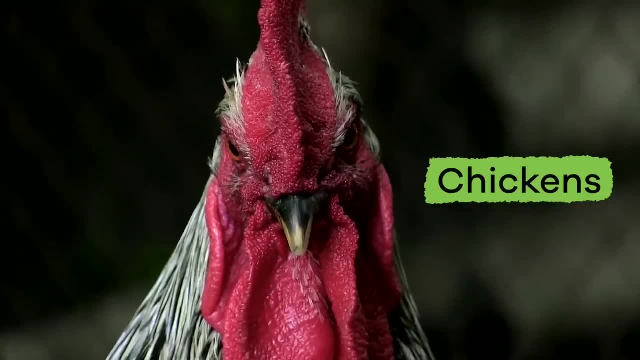 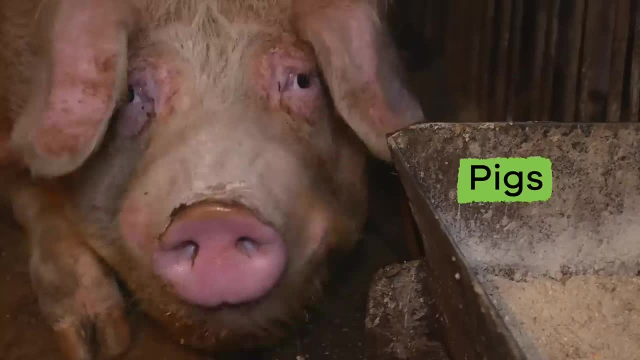 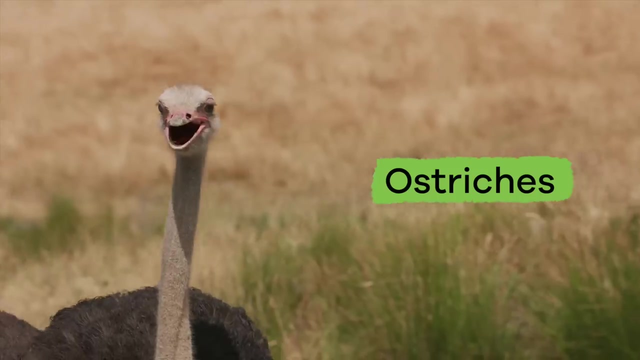 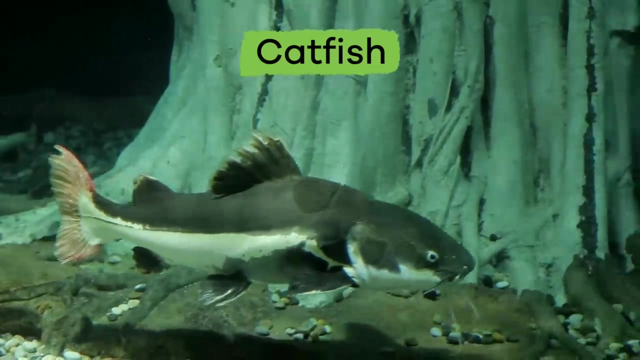 just like herbivores. Chickens, crows, bears, raccoons, skunks, pigs, robins, lizards, turtles, badgers, ostriches, ducks, flies and catfish are all examples of omnivores. 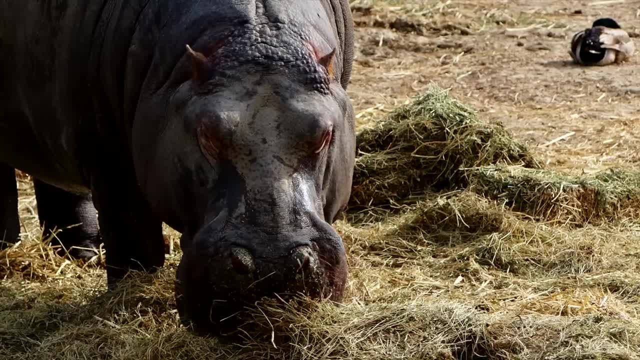 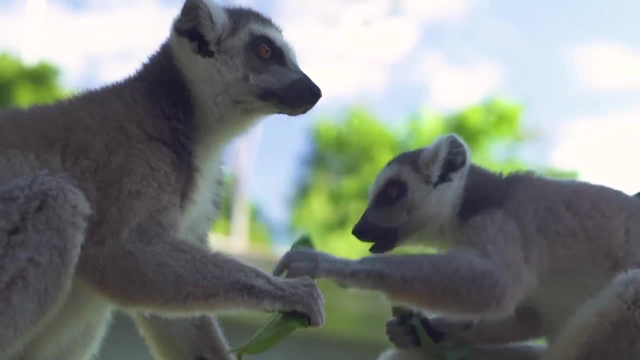 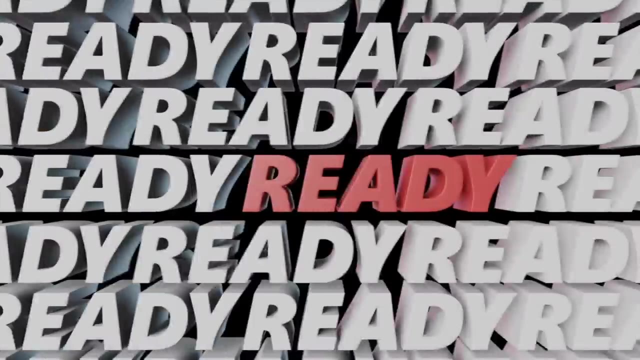 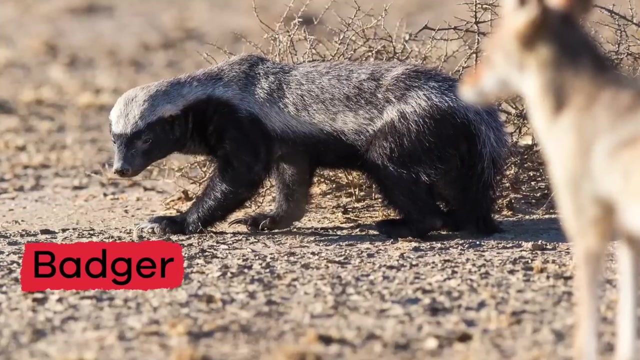 We are going to name an animal and you have to tell us if it is an herbivore, carnivore or an omnivore. Ready set go B. Herbivore Badger, Omnivore, Venus, Flytrap Carnivore. 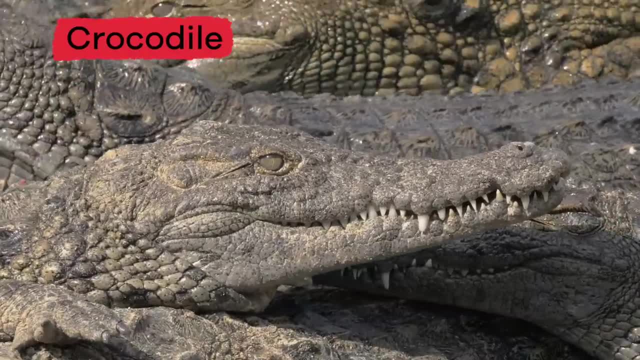 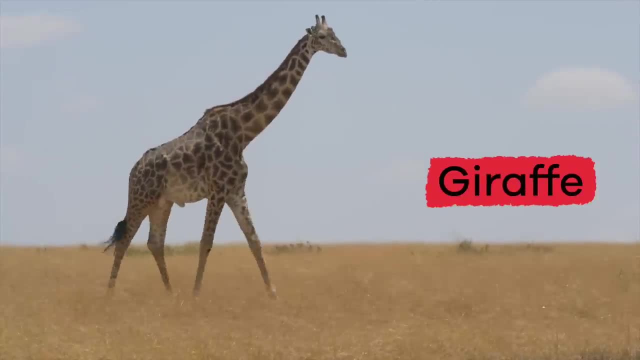 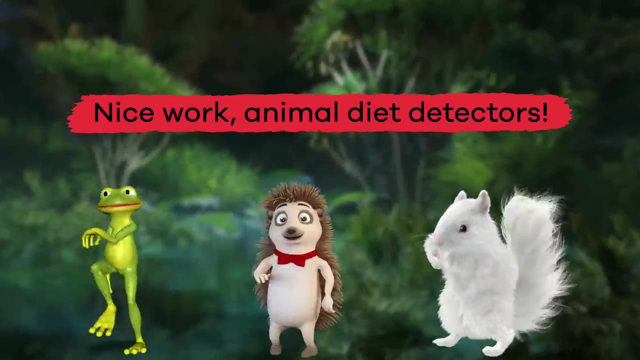 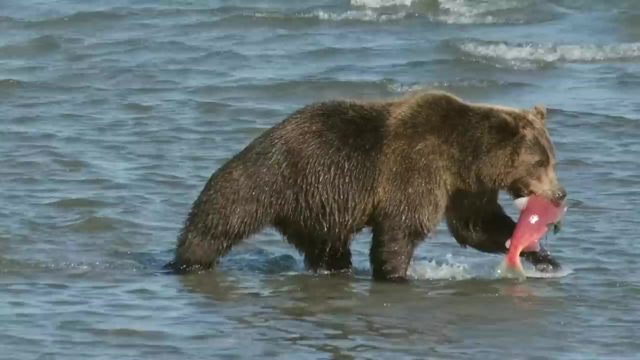 Crocodile, Carnivore, Parrot, Herbivore, Giraffe, Herbivore, Catfish, Omnivore, Nice work Animal Diet Detectors. Like humans, animals have all different kinds of diets, whether they eat plants, meat or a little bit of meat. 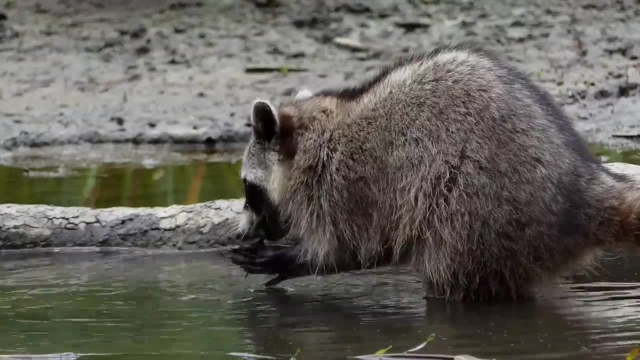 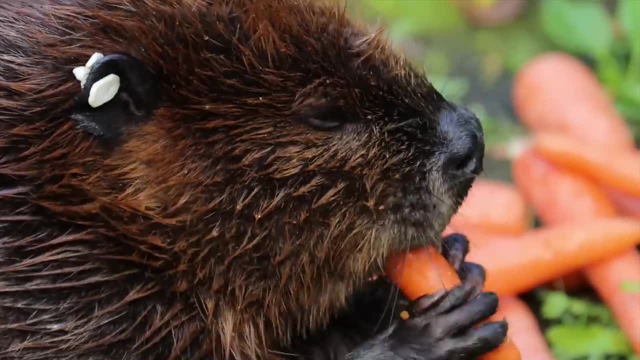 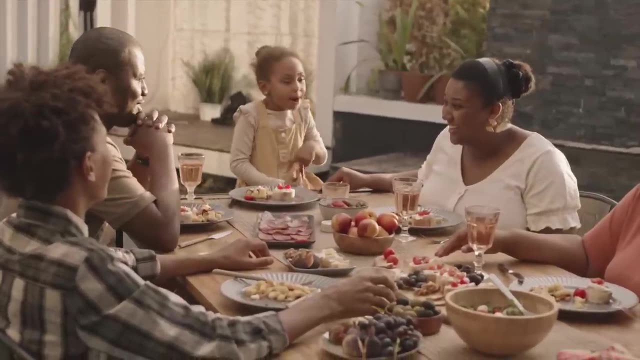 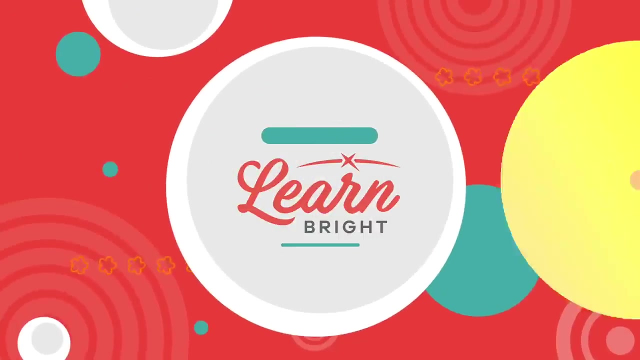 think about what parts of your meal herbivores, carnivores and omnivores would eat. You can even make it a fun game you can play with your family or friends. Hope you had fun learning with us. Visit us at learnbrightorg for thousands of free resources. 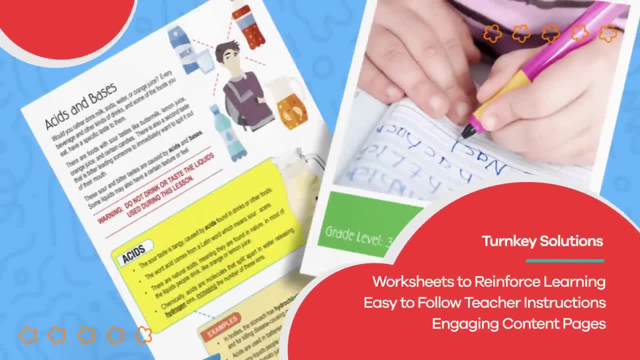 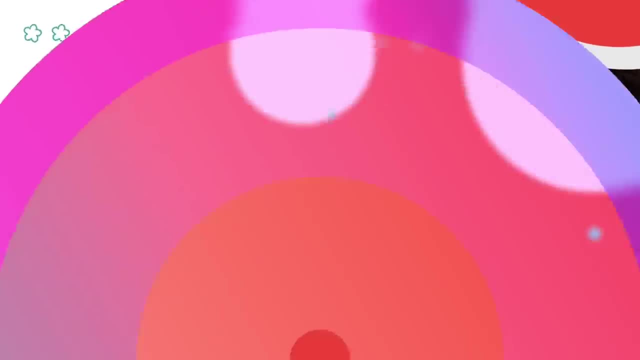 and turnkey solutions for teachers and homeschoolers. Learn more at learnbrightorg. 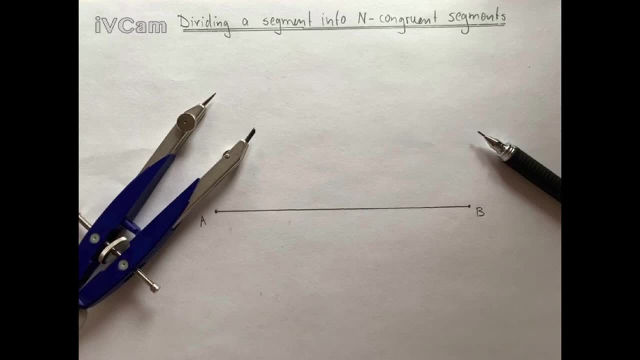 Okay, so in today's video, we'll be learning about how to divide a segment into n congruent segments where n could be any integer value or positive integer. Let's, for instance, take an n value to be equal to 3.. Okay, so how do we split this segment into exactly? 3 congruent segments. Okay, so, in order to do this, the first step and at some angle that is either above or below the line. Okay, so, I'm picking a line that goes above, like this: Okay, so, after drawing this line, we'll be taking our compass times, Okay. to point d and to point e, and we already know how to copy angles at this point. so first we draw an arc through any parallel lines here. okay, so the next step is to measure the distance between these two points here of the intersection of the arc and segments ac and bc. and you know once we measure. the distance. we can then copy the angle. okay, so we already learned this. that's just simply the copy angle method. okay, so here we draw an arc and then from this point we draw another arc here, okay, okay, wherever they intersect here, i will label this with a. point, and what we want to do now is connect points d or point d with this point here, like that. and then we want to connect point e with this point, like this, okay, and there you go. these lines now all parallel, okay. so i'm going to label these points now. let's label these points as f, g, and we have b already, and it turns out that segment ef is congruent to segment f- we discussed it here- and then these segments must be congruent as well. so why is this true? why does this construction work? okay, so the reason why it works: is because, um, since we copied the angles here, here we know that line, so let's write this here: we know that line BC is parallel to line DG and parallel to line EF. okay, why is that? why are these lines all parallel? well, the reason is because, you know, we can look at AC as the transversal, so we can.